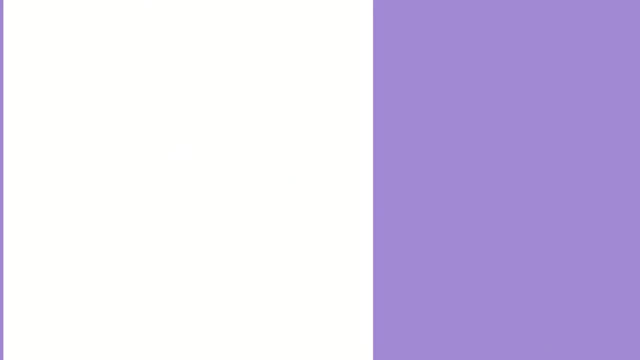 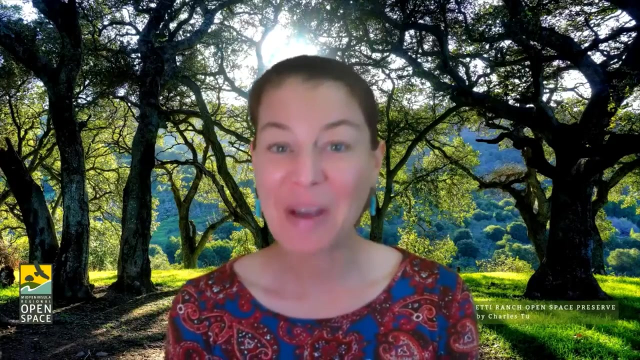 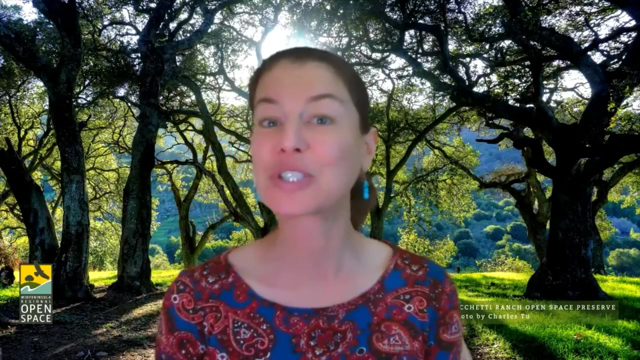 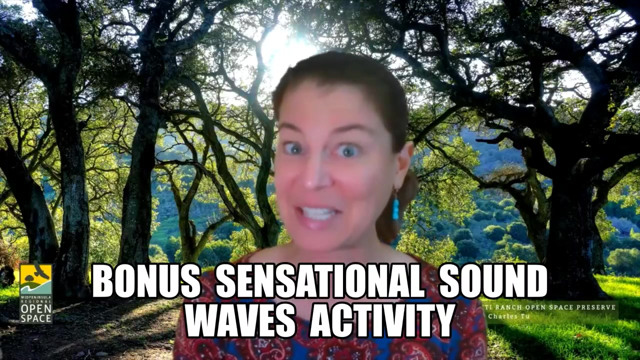 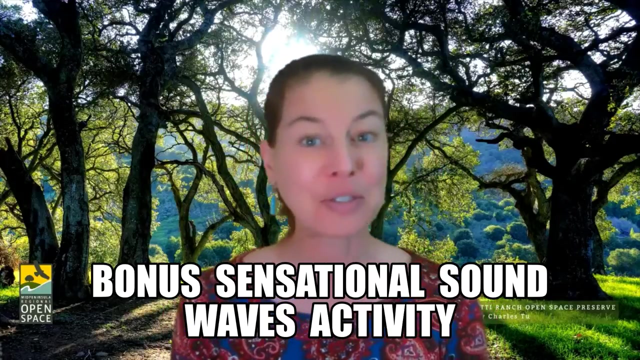 Hello my fellow scientists. Welcome to another episode of Science is Everywhere the home edition. My name is Marie Laika and I'm from the Children's Discovery Museum of San Jose, and I am back for a bonus Sensational Soundwaves activity. So we've already talked about what sound waves travel through solids, air liquid. We've also talked about pitch, high and low. 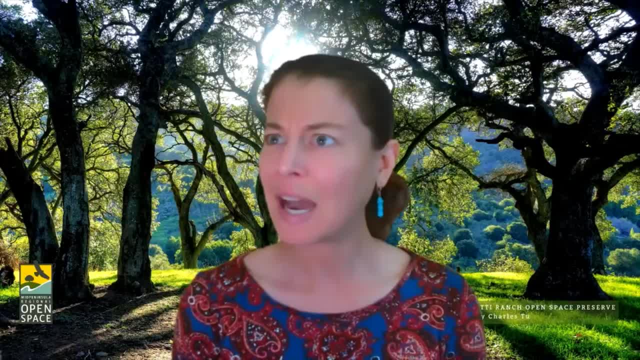 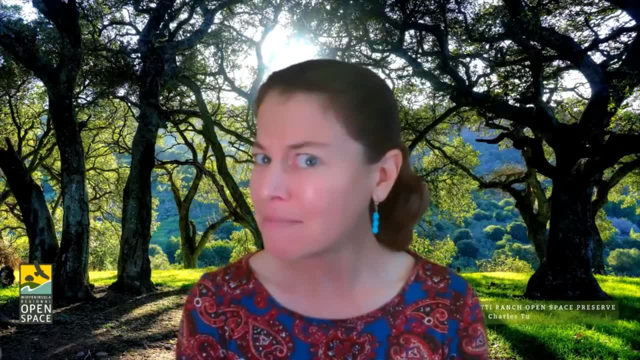 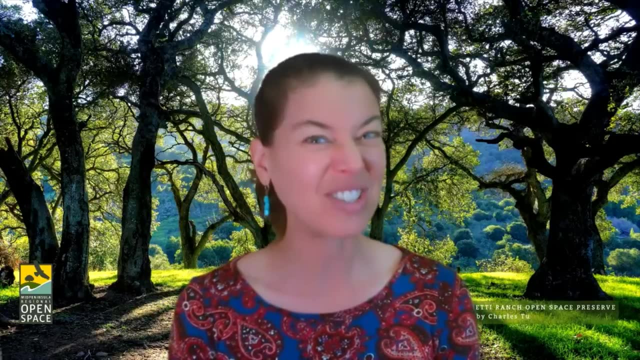 But I've had some scientists reach out to me and say: you know, how do we show that sound waves are real? We can hear them, but can we see them? And I thought, hmm, this would be a great opportunity to do a very simple experiment in order to actually see sound waves. 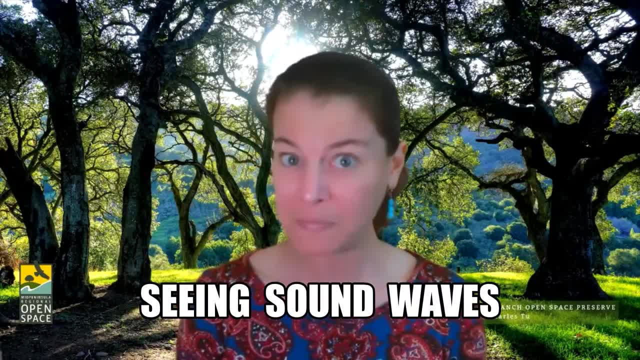 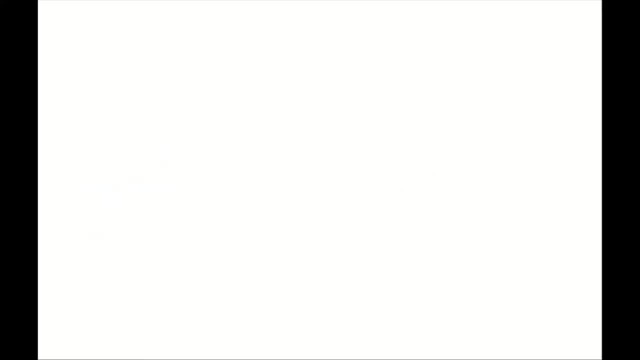 So let's do a quick review on how sound waves travel, and then we'll set up the experiment And then I'll show you how you can actually see sound waves. So for our quick review on how sound waves travel, I'm going to use a lovely bird we had outside of the window this morning. 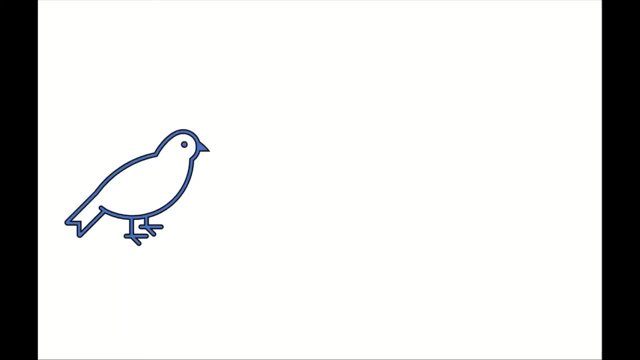 There you go. So the sound that the bird was making was traveling. It was traveling by waves or vibrations through the air to me and my ear, so I could hear them. Okay, so now that we've reviewed that, let's go ahead and set up our experiment. 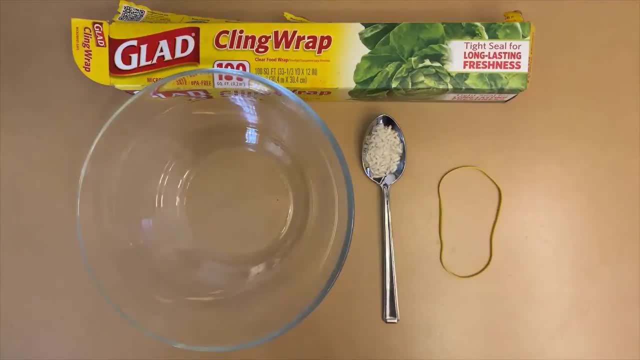 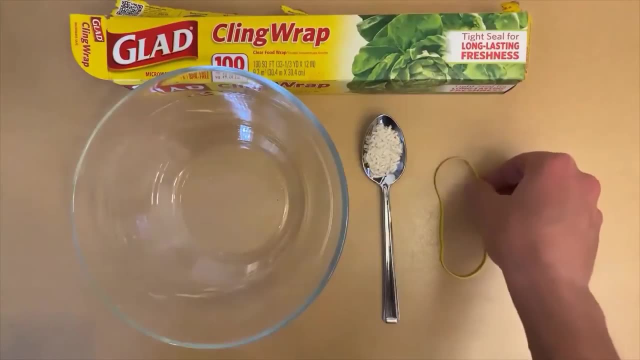 This is all we're going to need for this experiment: A bowl, Some plastic wrap, A rubber band And some small dried objects. I've just got some rice. You can use confetti, You can use dried beans, Just something that's about that size. 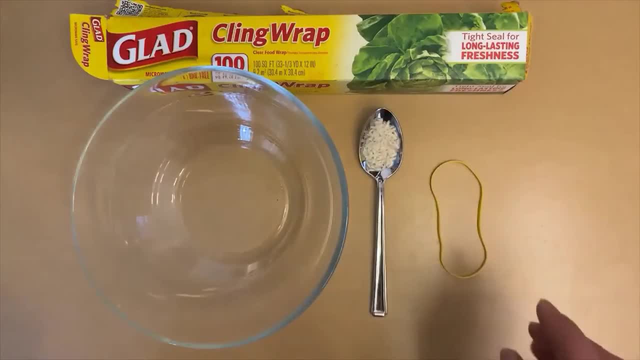 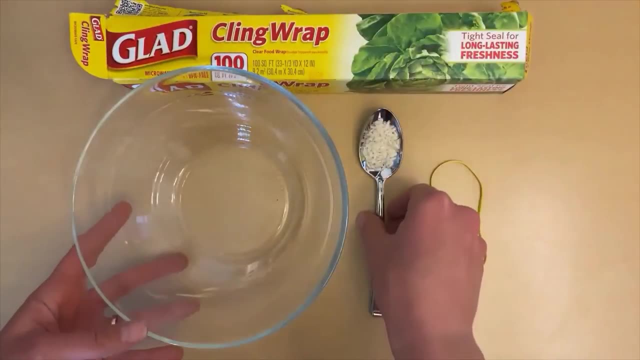 And I'll show you how that works in just a second. So first thing we're going to do is we're going to work with our plastic wrap and our bowl and a rubber band to set up the base of this experiment. So I'm going to move my little objects out of the way so they don't end up going everywhere. 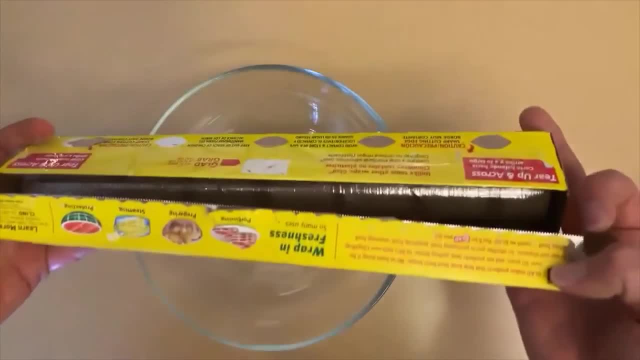 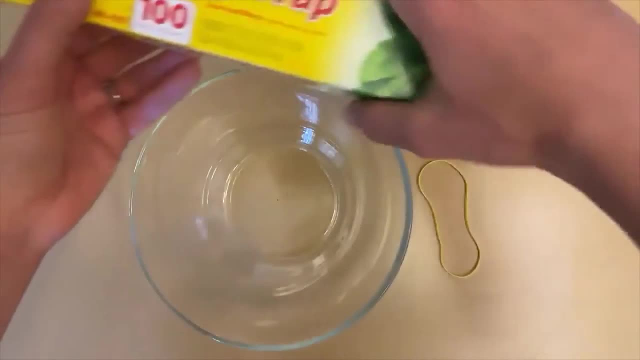 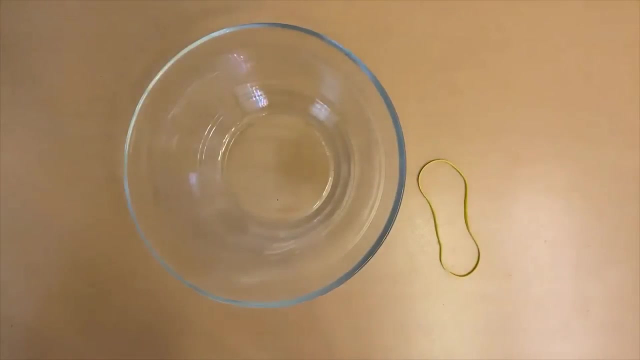 And I'm going to go ahead and take a sheet of the plastic. pull this out enough to cover the top. Okay, Once I have that, go ahead and take that piece of plastic And if you're using cling wrap, remember it does have a personality. 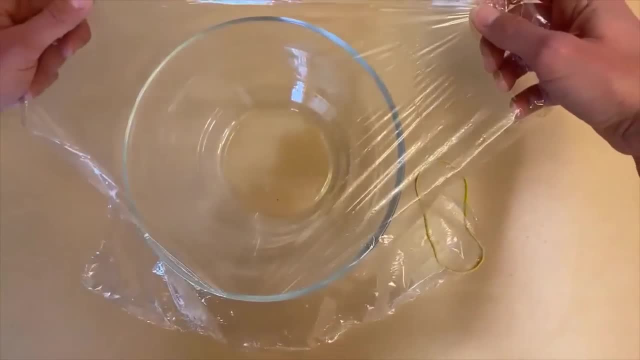 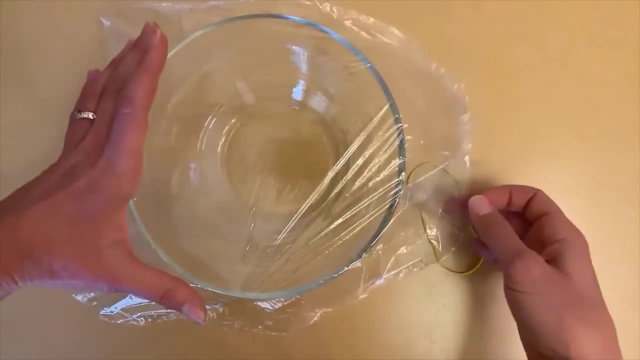 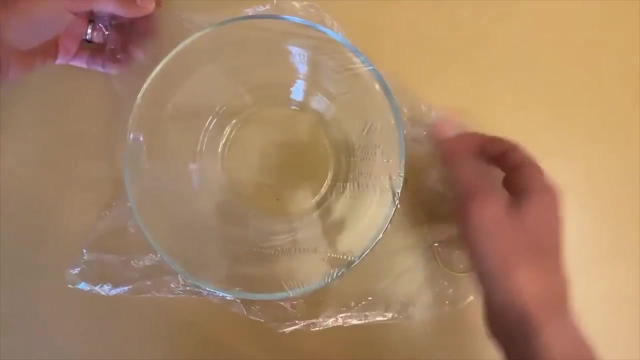 So just be patient with it The best you can. you want to pull it, so it's pretty tight, You don't see any wrinkles, Or again, at least the best you can. The tighter you can do this, the better the experiment's going to look. 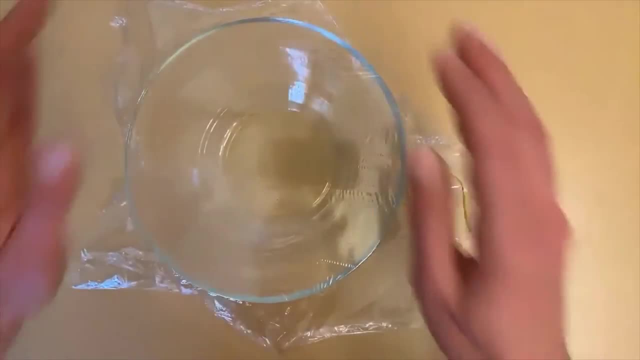 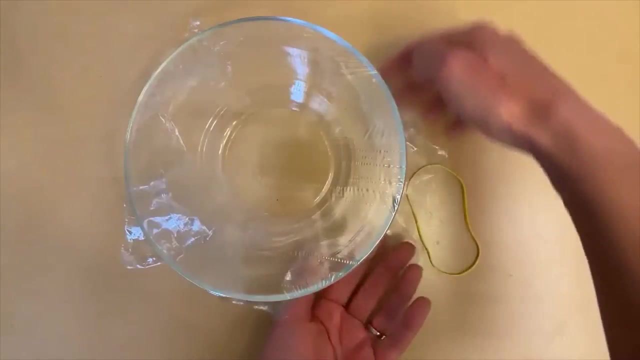 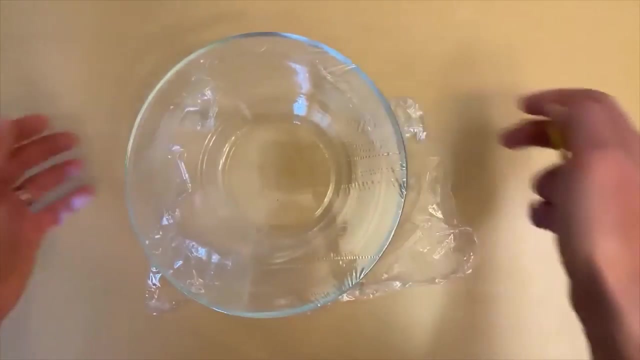 It's got a little bit of a wrinkle- No big deal. Gently tuck it down, And you also want to make sure that you don't tear it. So that's, you got to be gentle. Okay, Then, if you've got cling wrap sometimes, that's okay and that'll just cling to the sides and be all right. 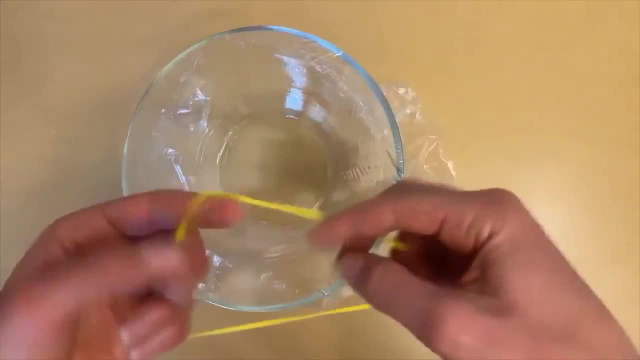 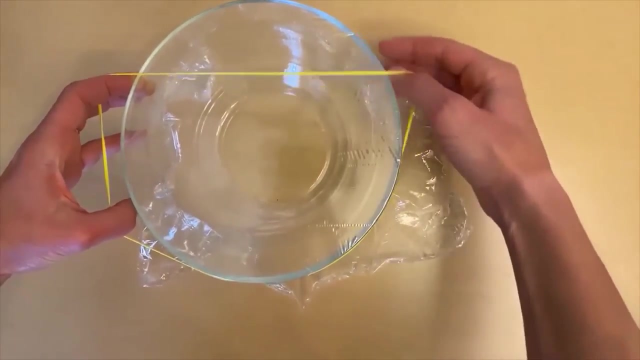 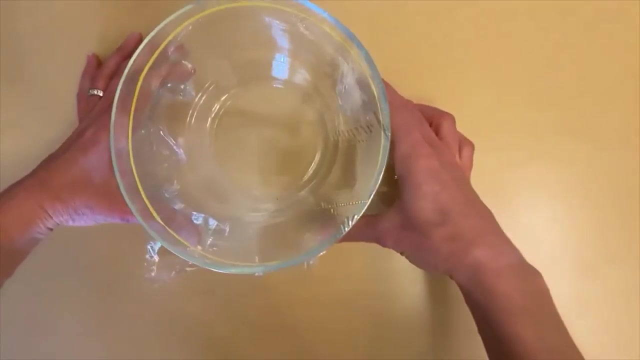 If you're using any other type of plastic, that's where this rubber band can come in handy. What I'm going to do is go along the outside of the bowl Again, really gently- Don't want to tear that. That'll help hold that where I want it. 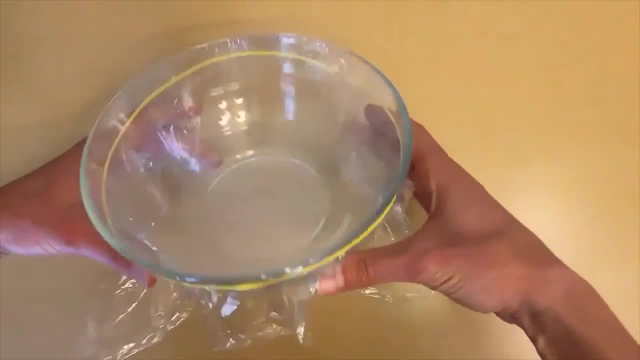 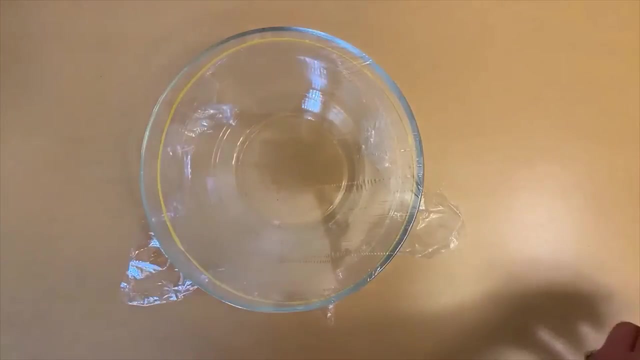 So if you take a look, I'll look from the side Just like that, Okay, And once you have that set up, looks like a little mini drum. you're going to take your small objects, Bring those back in the spoon. 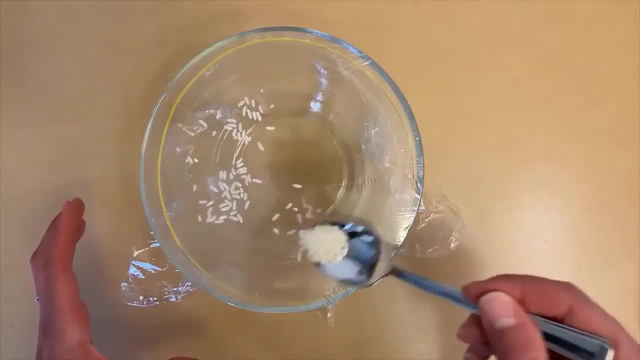 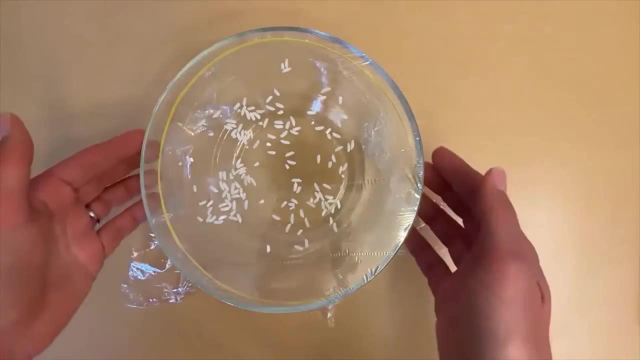 And just sprinkle a few on the top, Just like that. And that's not an exact measurement. You just want to put a little bit on the top. And now you are ready for the next stage of the experiment: to see invisible sound waves. 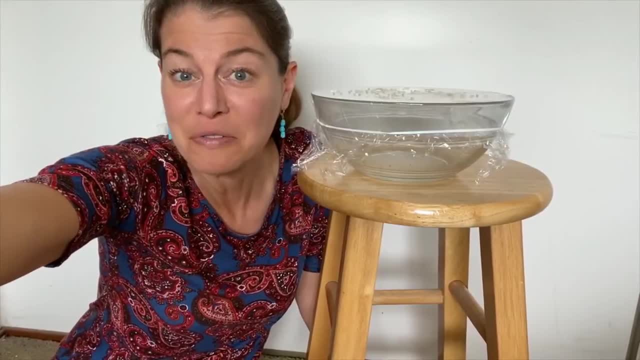 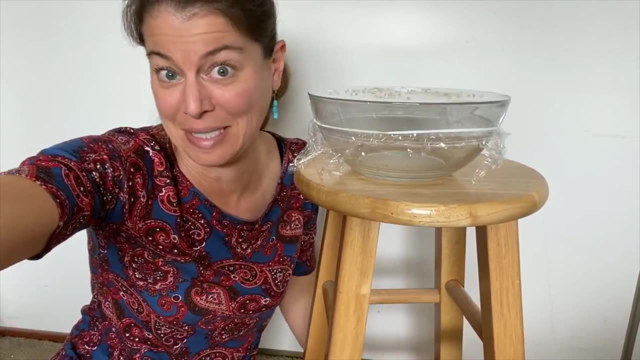 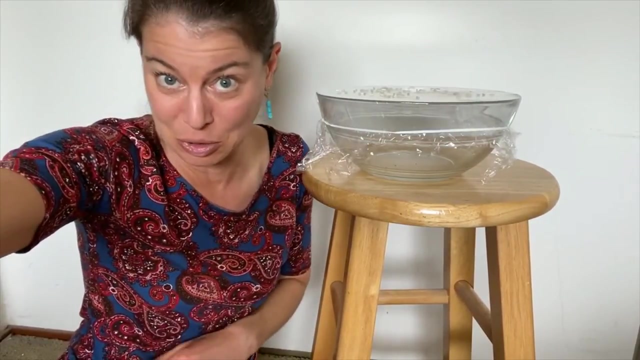 Okay, I moved our experiment to another room And I put the bowl on a stool And I am actually sitting on the floor. And the reason is is because, first of all, I wanted you to see that I am not going to be touching the stool. 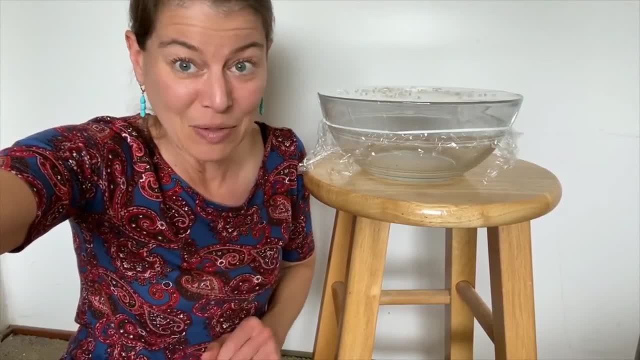 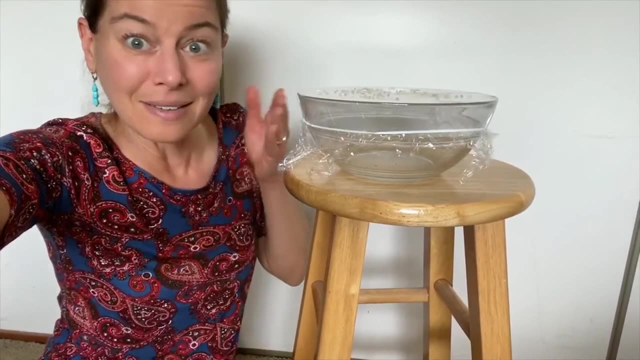 I'm not going to be tapping on the bowl or anything like that. Second thing is, I'm going to need to get really close to that bowl in order to make a sound, but still not touching it. So I just wanted to make that a little bit easier. 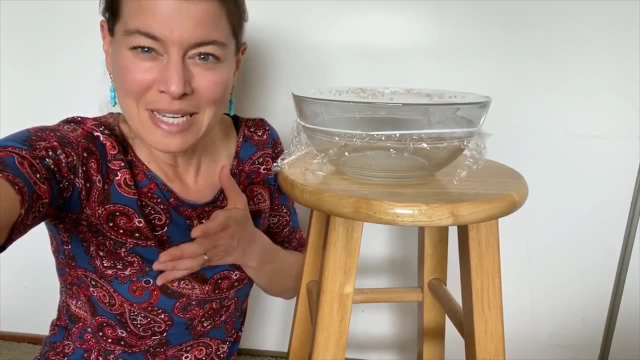 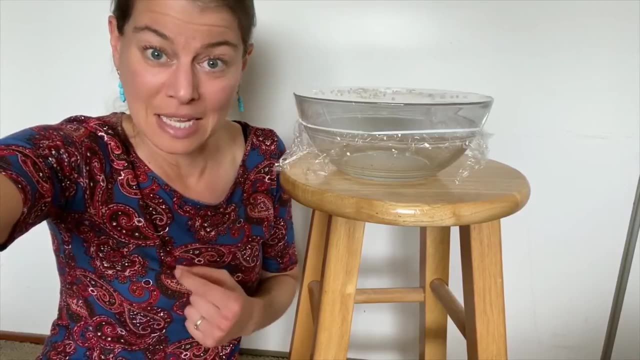 So I just wanted to make that a little bit easier to see. So what am I going to do for a sound? Well, it's really easy for me to hum. So I'm going to pick a pitch and I'm going to hum and see if I can make those grains of rice move. 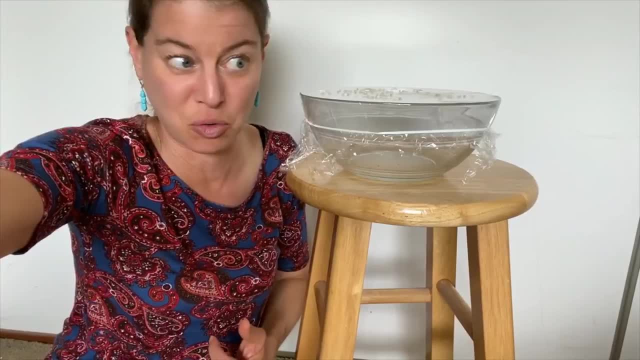 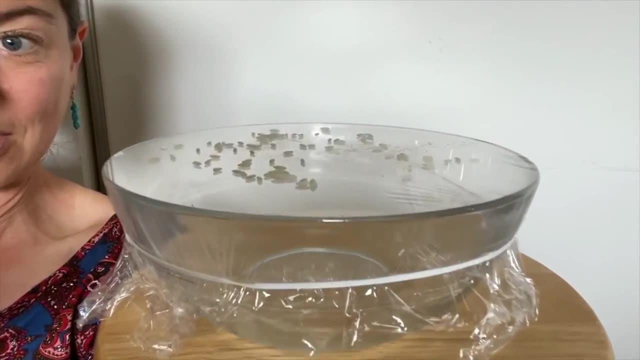 Therefore, kind of showing how a sound wave is traveling. Okay, so I'm going to have to get you close and get into your personal space, So hold on, Here we go. I'm going to get you close so you can see those grains of rice. 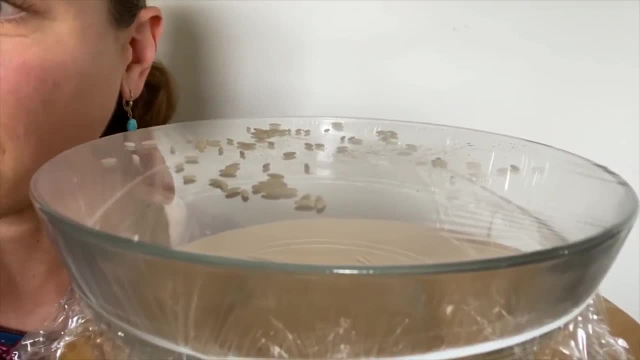 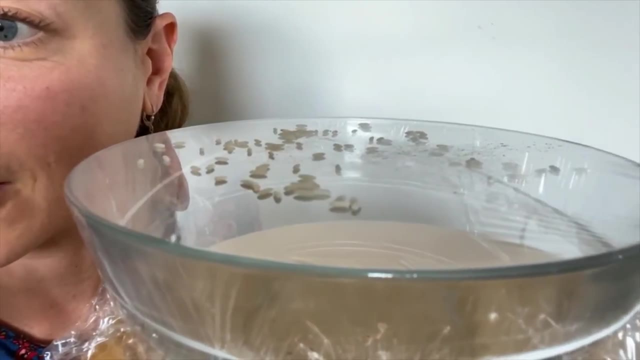 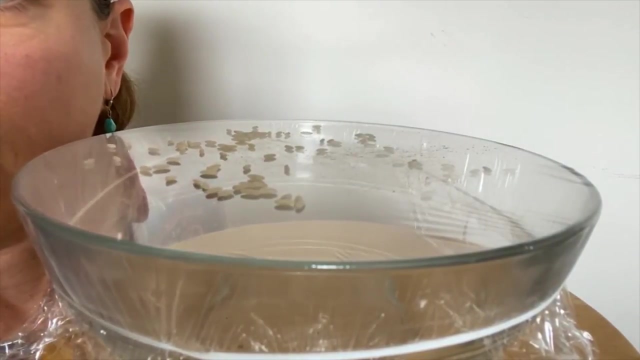 Okay, Now I'm going to put my face right up here and you take a look, I'm not touching. I'm close, but not quite. Okay, Go over here, Pick a sound And here we go. Did you notice something? 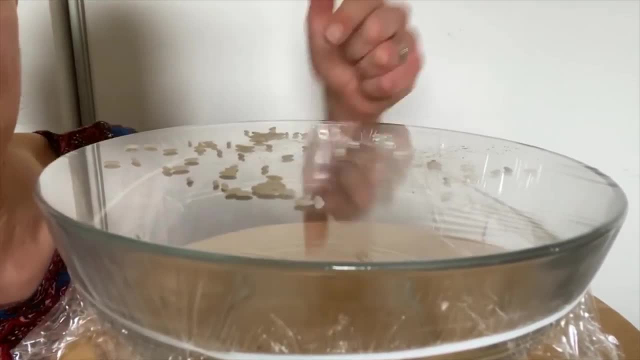 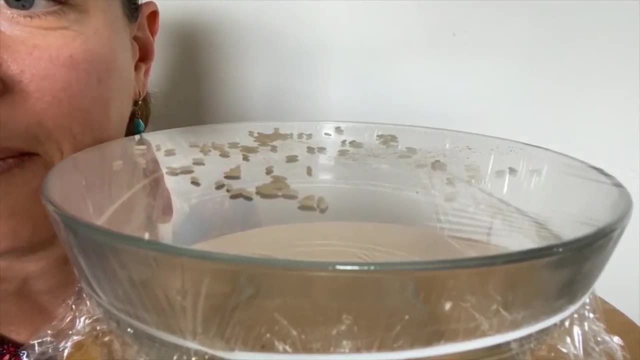 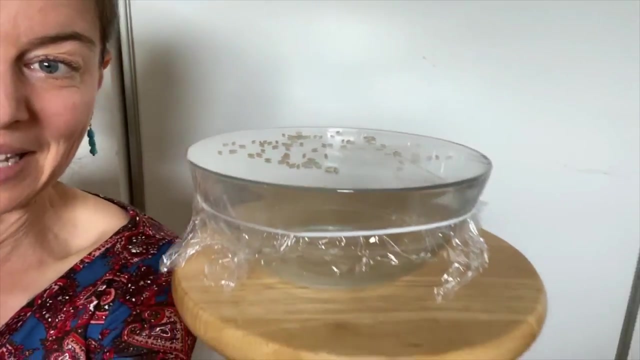 Let's try it again and pay attention, moreover, to like the grains of rice. They're a little bit closer. Here we go. Looks like they're kind of dancing, right, Okay. So let's back you up a little bit and let's talk about it. 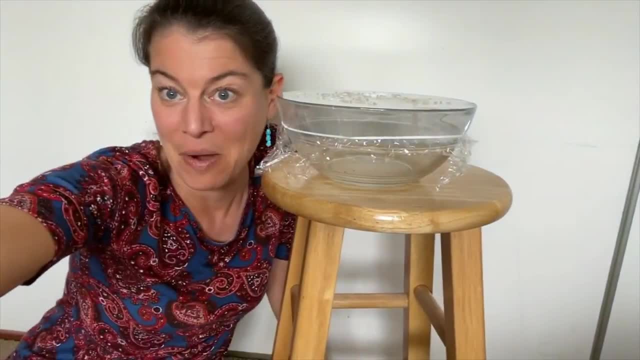 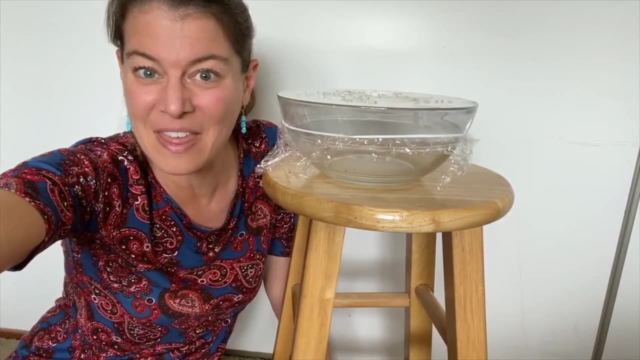 Why did that happen? Well, we've been talking about how sound waves are invisible, right? Well, even though they're invisible, they are still there and they're vibrating. They're vibrations, So they're traveling through different things, like air and water, which we just talked about. 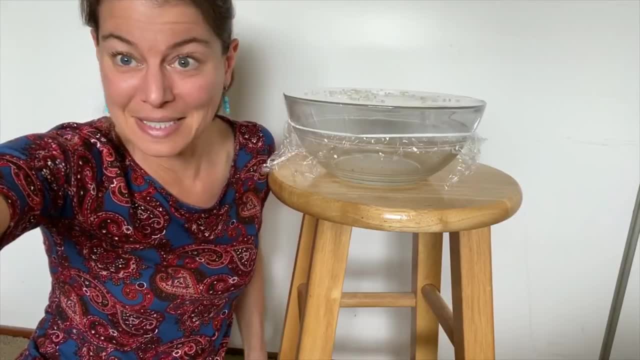 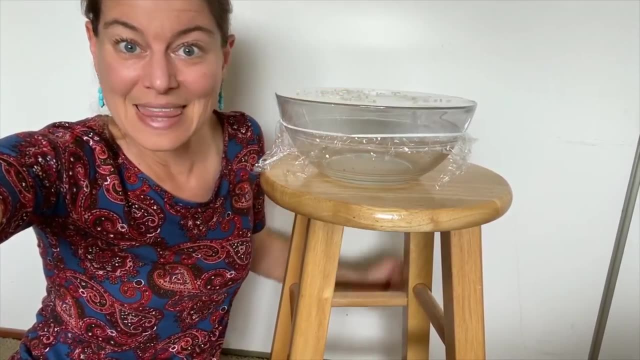 Like air and water, which we did earlier this week. Well, in this case they're traveling from me through the air, into the bowl, through the plastic, and then into the grains of rice which are then hopping. It's vibrating, all those different things. 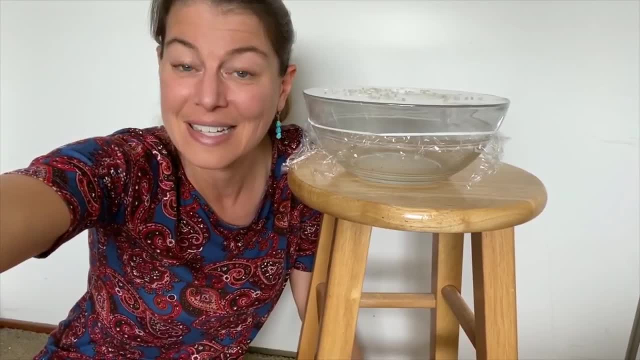 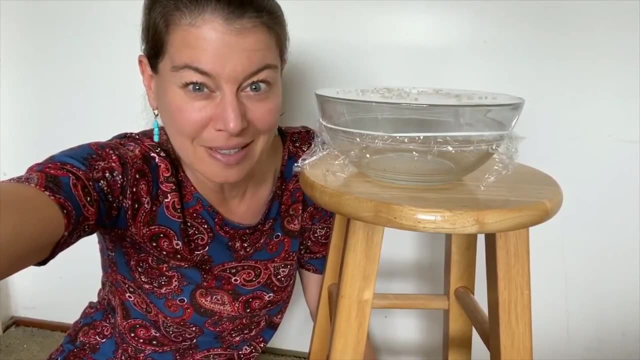 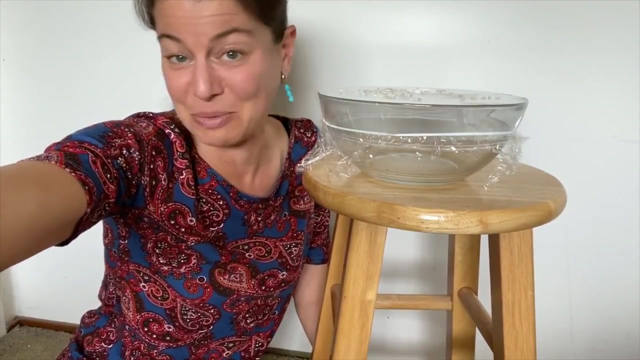 And that's the way you can see sound is through those vibrations and how things change. Fun bonus activity: Pick your favorite song, Turn it up, See how it impacts those little pieces of rice or solids or beans or whatever you have there. That's really fun to try.